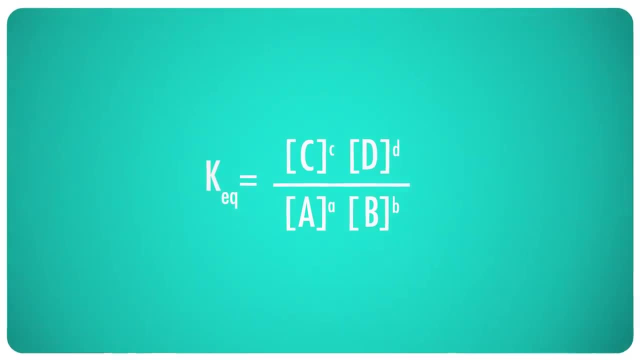 divided by the product of the molar concentration of the reactants, Each concentration isthen by A is raised to the power of its coefficient in the balanced equation. Now, this is important. We're using the coefficients as exponents here because we're multiplying all the products. 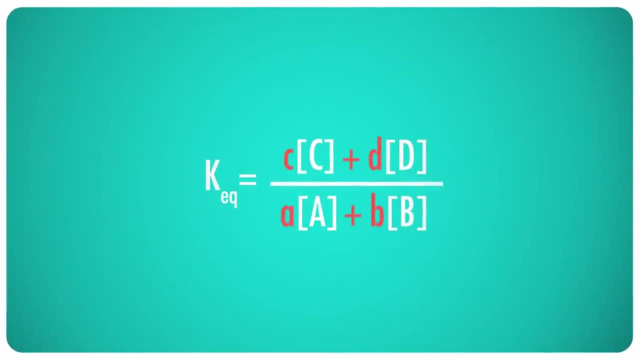 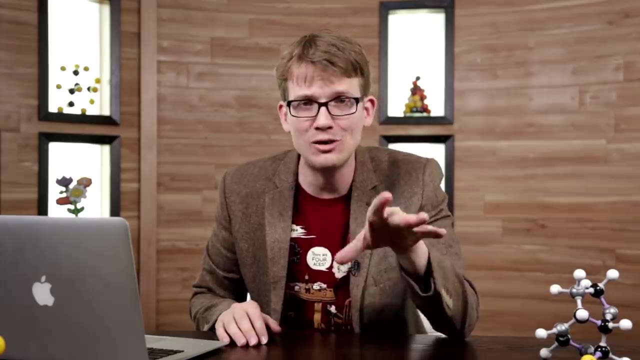 and all the reactants, not adding them like you would do in the balanced equation. Generations of students have messed up test scores by getting this part wrong, but you will not do that. So again, it's the product of the products over the product of the reactants and the. 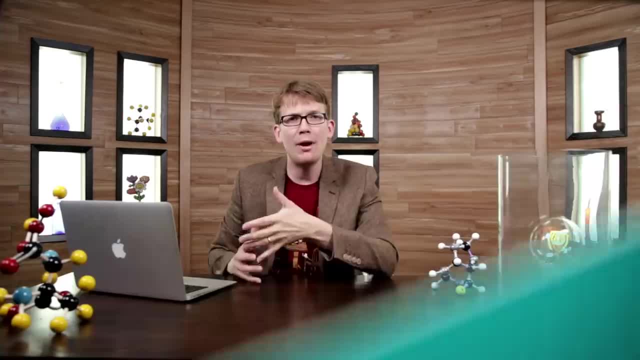 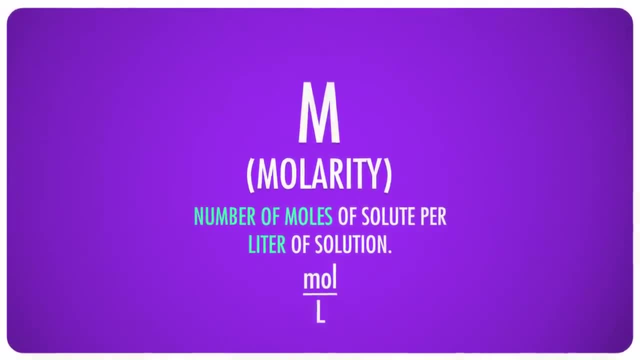 coefficients become exponents. Actually pretty simple. The square brackets in the formula are used by chemists to represent molar concentration or molarity moles of solute per liter of solution. These equilibrium constant equations and the constants themselves are one of the few places 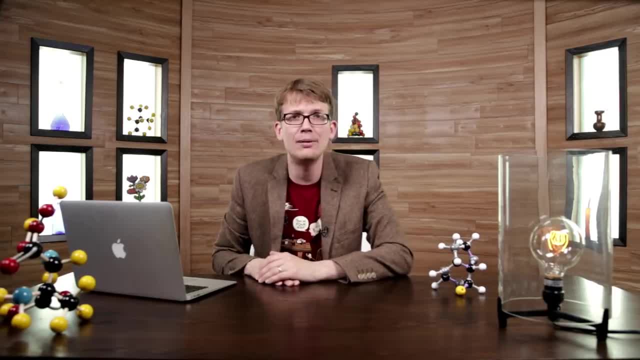 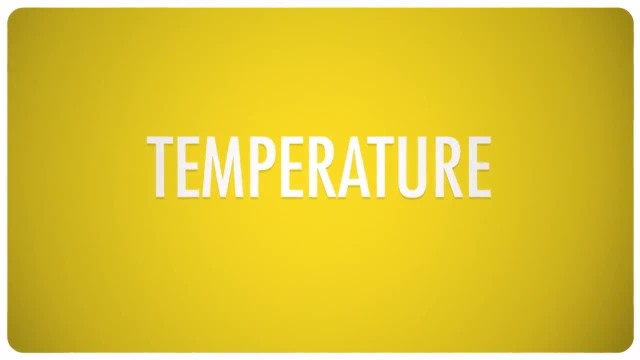 where you don't need to write them with every number. Just remember to convert everything into molarities before plugging numbers into the equation. One last thing before we do a calculation. As we learned in the last episode, a change in temperature changes the position of equilibrium. 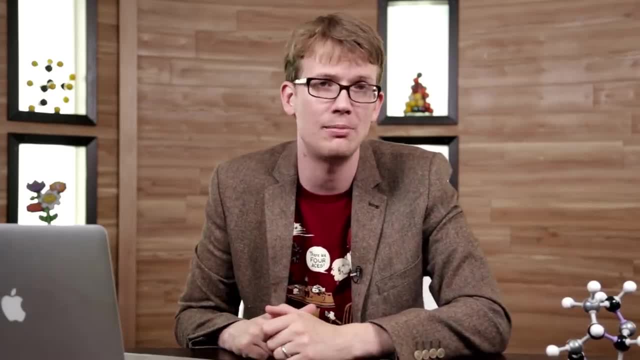 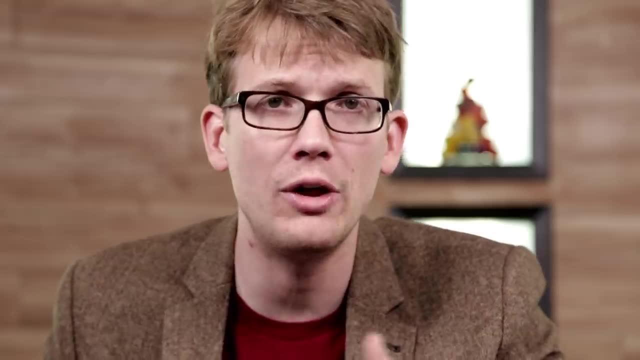 Therefore, the equilibrium constant is only true for a specific temperature. Constants are normally calculated at 25 degrees Celsius. This is close enough for most situations, but the temperature should always be mentioned along with the constant. Fortunately for us, chemists have already figured out the equilibrium constants for. 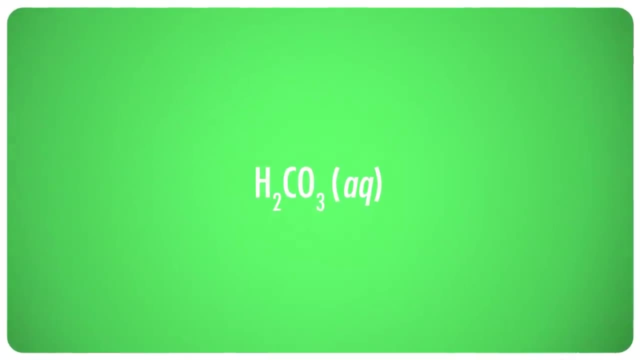 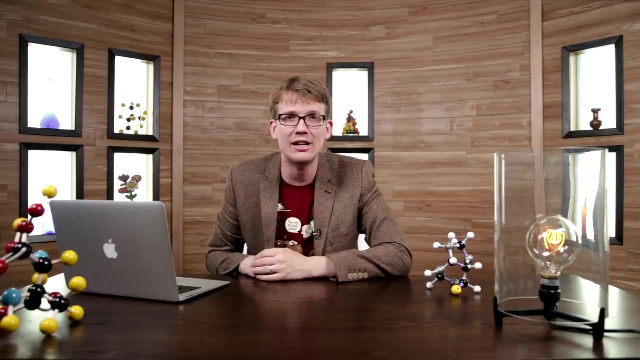 most common reactions. Carbonic acid, for instance, which is basically just carbon dioxide dissolved in water, dissociates to form carbonate ions and hydrogen ions. You'll see this reaction again later when we talk in-depth about carbon and the planet's carbon cycles. 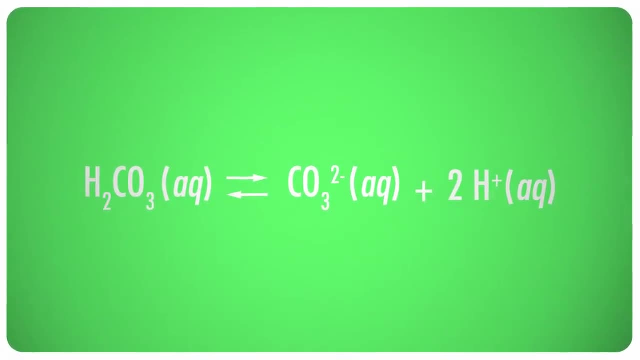 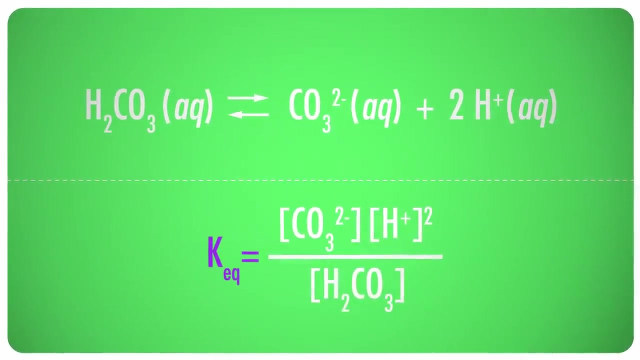 More importantly, right now, the reaction is perfectly reversible, with an equilibrium constant of 1.66 times 10 to the negative 17th. That's a lot. That's a lot For this reaction. Keq equals the product of the molar concentration of the carbonate. 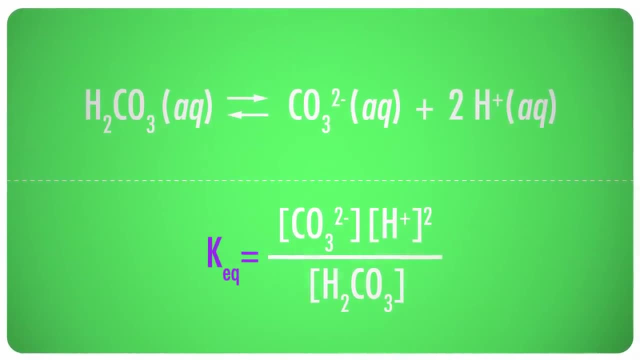 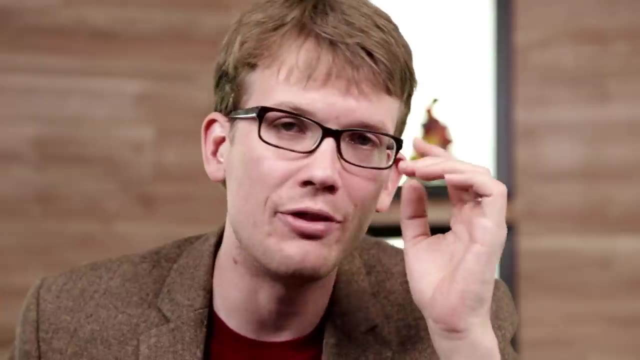 ion and the molar concentration of the hydrogen ion, which is squared, because hydrogen's coefficient in the balanced equation is 2, all divided by the molar concentration of carbonic acid. Now let's not be boring and throw a bunch of numbers around. 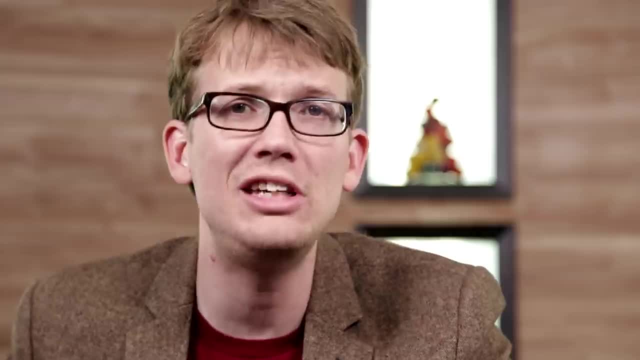 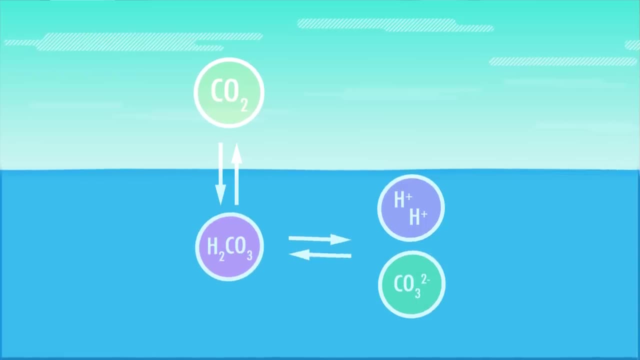 What you need to see is that the quotient on the right must always yield the same number, because it's a constant. So if the amount of CO2 in the atmosphere increases, leading to more H2CO3 in the Earth's water, The concentration of carbonate ions and or hydrogen ions must also increase, so the total 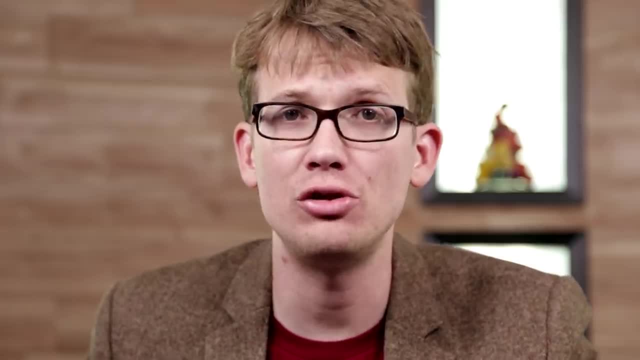 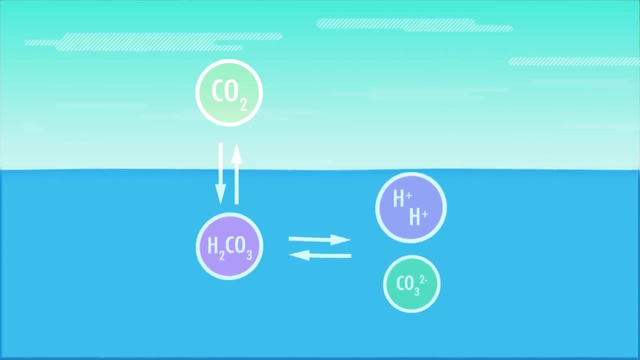 will match the Keq. You should also notice that any change to the concentration of hydrogen ion will have a huge effect on the denominator because it's squared. So an increase in hydrogen ions, like if the water were somehow acidified by an outside. 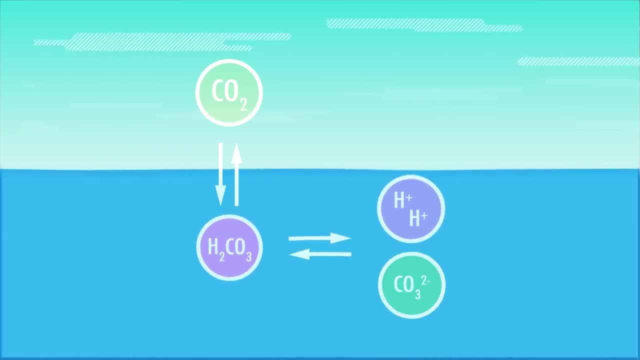 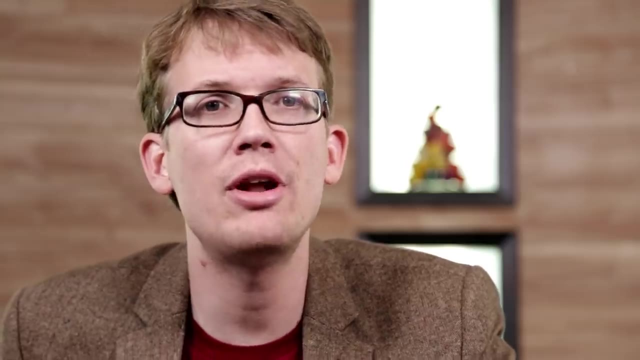 source would require a huge decrease in carbonate ions or a huge increase in carbonic acid, carbon dioxide, pulled in from the atmosphere to satisfy the equilibrium condition again. We can attack this problem from another direction too, Depending on what it does. 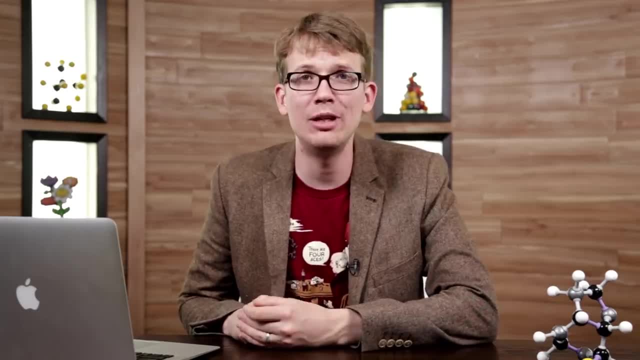 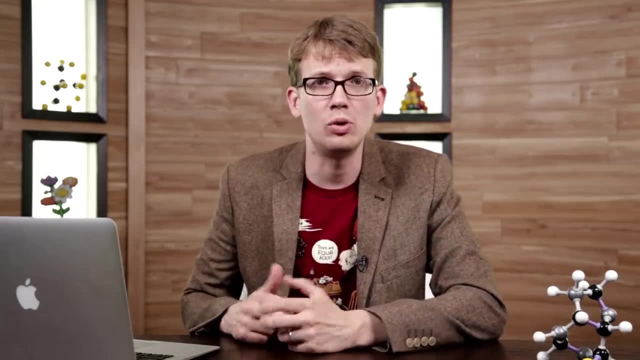 What information we have to begin with, Chemists often know not only the equilibrium constant for a reaction, but also how much of each reactant is available, And all they need to figure out is exactly how much of each substance will be present at equilibrium. 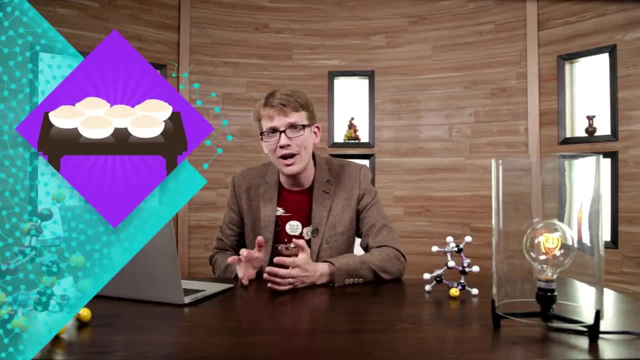 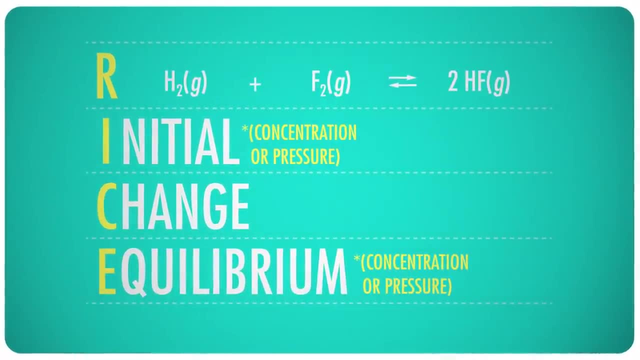 This type of calculation is easiest using a format called a RICE table. RICE stands for Reaction, Initial Change and Equilibrium. On the R line at the top of the table we write the chemical equation of the reaction, leaving space between each part. so we'll have room to add more information below. 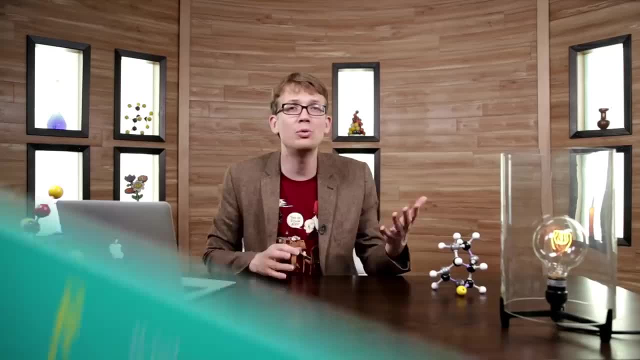 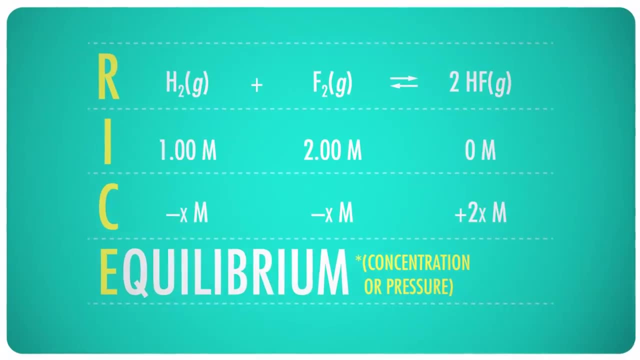 On the I line we write the initial concentration. Some of those will almost always be zero, since products generally aren't present until the reaction begins. The C line is where we map out how much of each substance will change during the reaction. We often don't know exactly how much this is until we do the math, so we start out with. 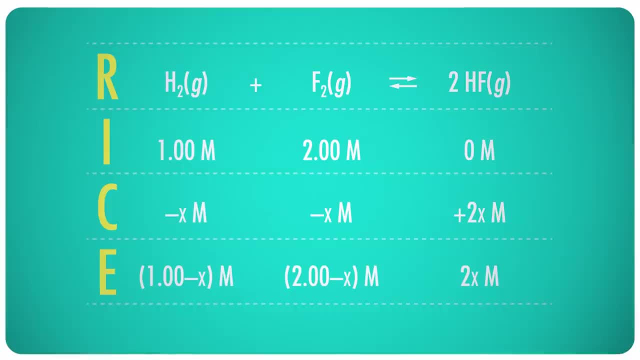 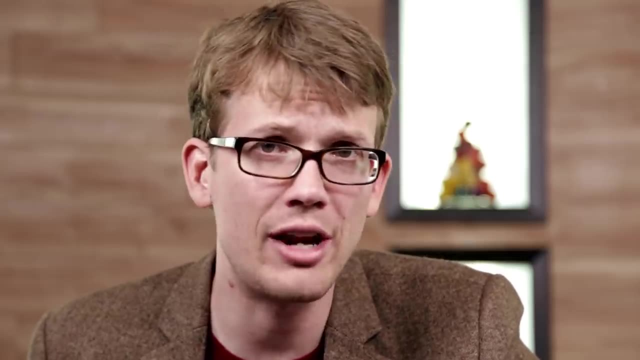 X, where the amount is unknown. The E line is where we put the final result: how much of each substance will be present at equilibrium, Since the final amount is just the initial amount plus any changes that have occurred. this line is the sum of the initial line and the change line. 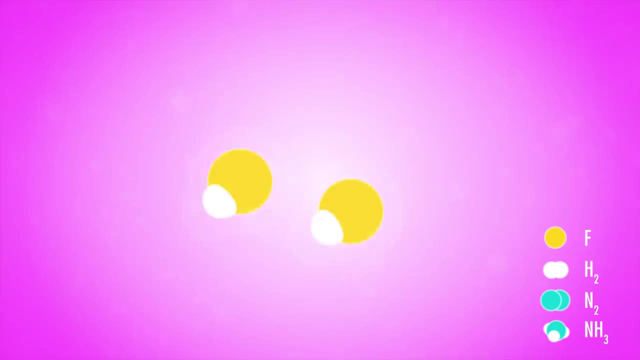 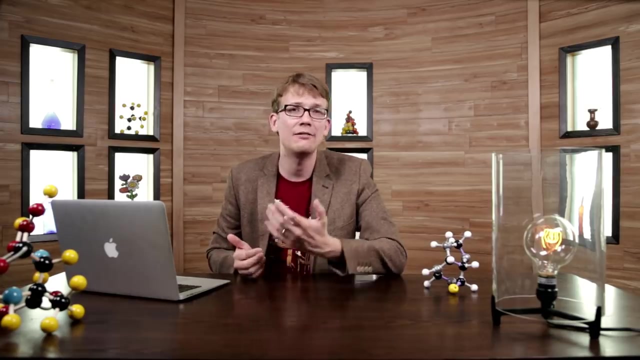 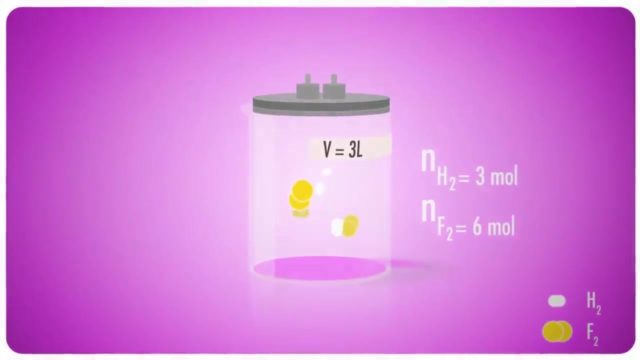 Let's do this for hydrogen fluoride or HF. an integral part of the process of refining gasoline, It can be formed in the gaseous state by an equilibrium reaction between hydrogen gas and fluorine gas. Start by writing the balanced equation For our initial concentrations. let's use 3.00 mole of H2 and 6.00 mole of F2 in a 3.00. 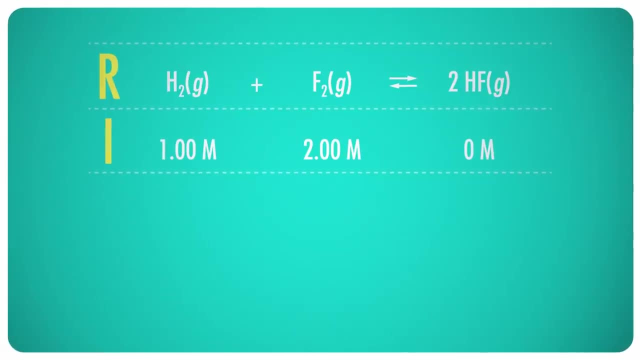 liter container at a certain temperature. That makes the initial concentration of H2 3 moles in 3 liters or a 1 molar solution. Similarly, the initial concentration of the F2 is 3 moles in 3 liters or a 1 molar solution. 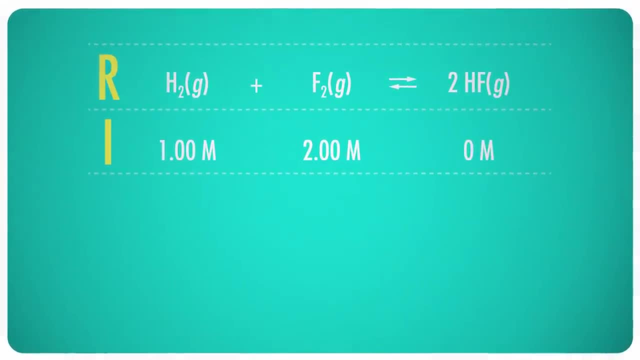 Similarly, the initial concentration of the F2 is 3 moles in 3 liters or a 1 molar solution. Similarly, the initial concentration of the F2 is 6 moles per 3 liters or 2 molar. 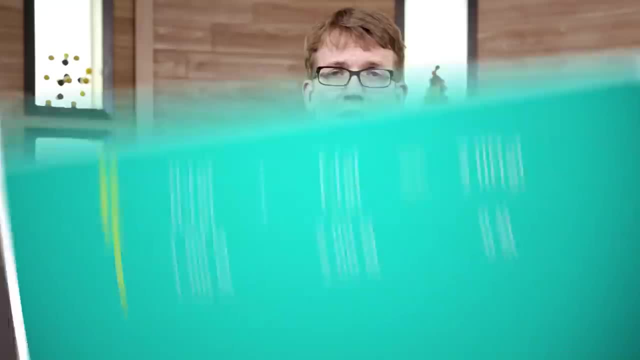 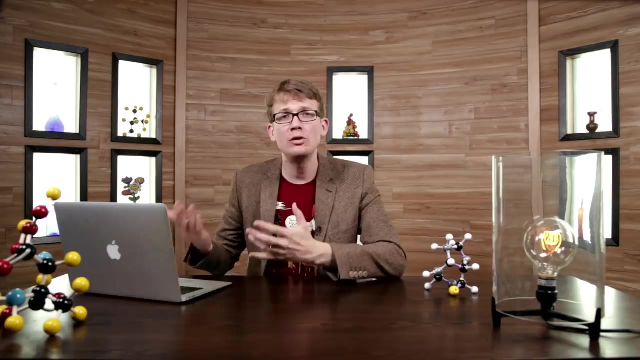 No HF has formed yet, so its initial concentration is 0.. So what we're trying to figure out is how much of the hydrogen or the fluorine will react to form hydrogen fluoride under these conditions. So we'll call the change x for now. 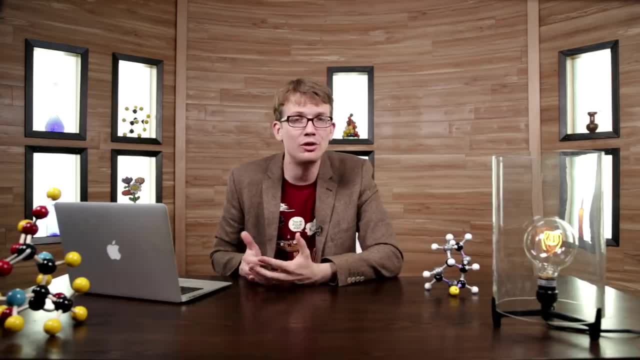 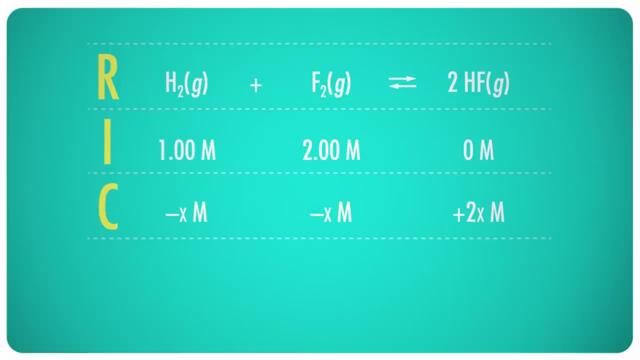 Since 1 mole of H2 and 1 mole of F2 combine to form 2 moles of HF, we can say that the H2 and F2 will each lose x moles per liter, while the HF gains 2 x moles per liter. 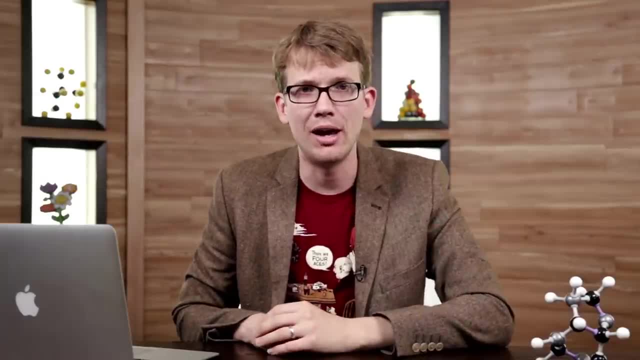 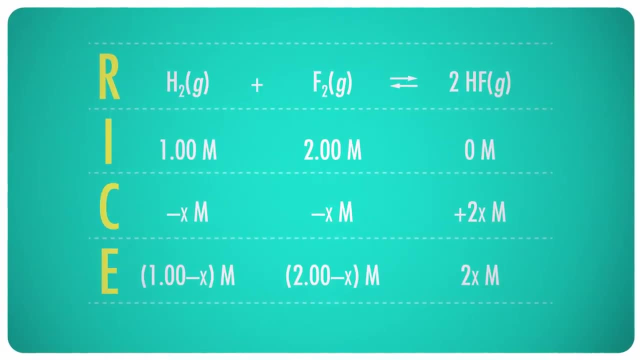 That's on the change line of your table. So that leaves the equilibrium line. Let's go back to the equation. You write your totals: For H2, we have a total of 1.00 minus x molar. For F2, the total is 2.00 minus x. 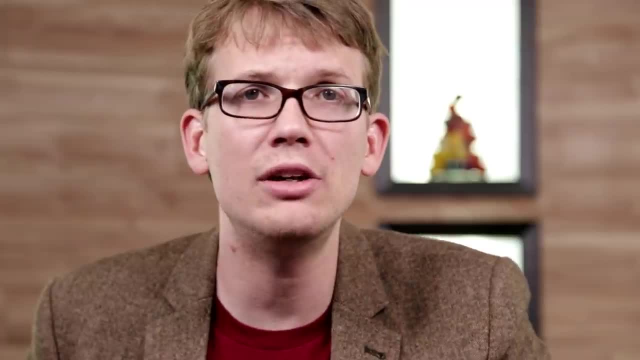 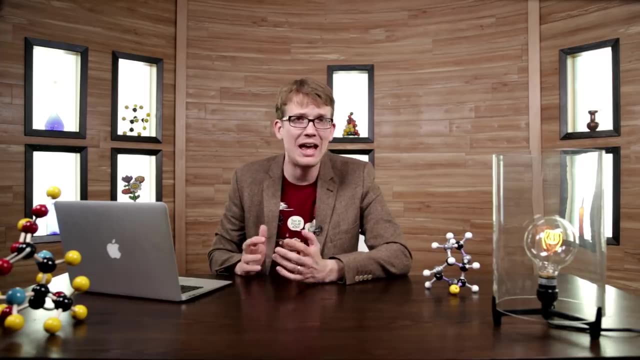 And for the HF the total is 2 x molar. Now we apply these figures to our formula for the equilibrium constant Based on the table in the back of my textbook. the Keq for this reaction is 115 at the given temperature. 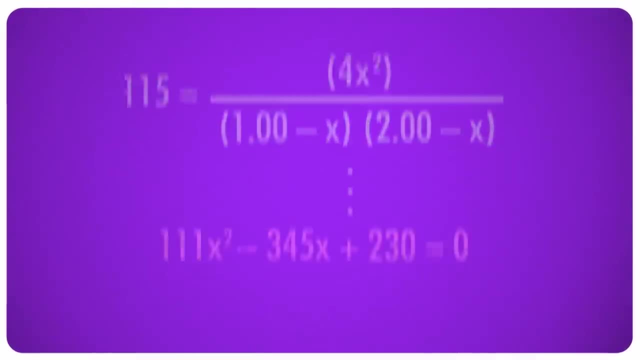 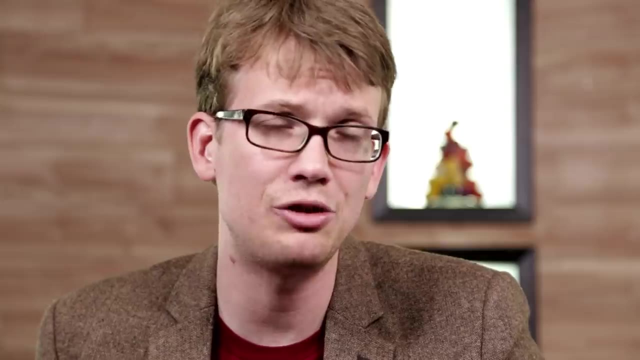 We plug in the numbers from our rice table and solve for x, and we end up with this, which you probably recognize as a quadratic equation. Just so you know, that doesn't happen with every equilibrium calculation, But it's an extremely common result. 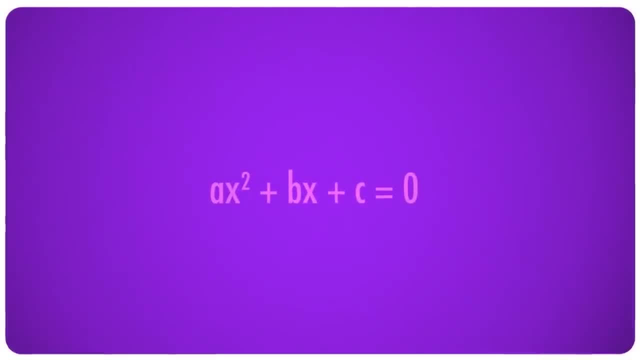 To solve the quadratic equation we have to use the quadratic formula, And to do that we have to think of the coefficients of our equation as a, b and c, in that order. Then we plug them in the corresponding positions in this formula: negative b plus or minus. 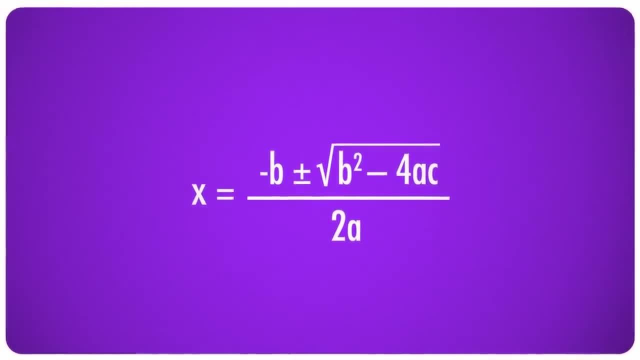 the square root of b squared minus 4ac, all divided by 2a. Once we finally get all the numbers in the right places, it becomes a matter of grinding through some basic algebra And, because of the way the quadratic formula works, we'll get two possible answers. 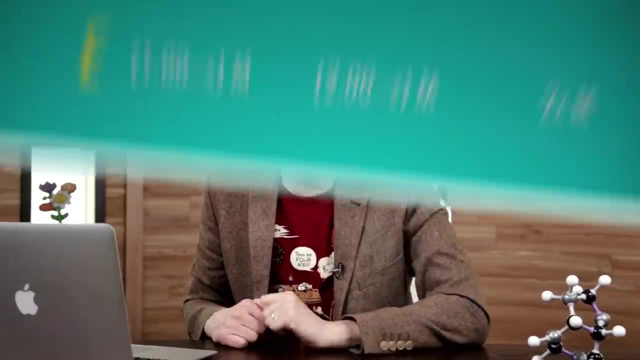 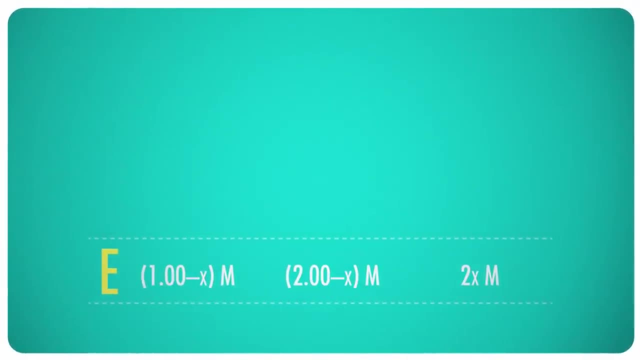 To figure out which answer is the right one. think back to the beginning of the problem. I said the initial concentration of the H2 was 1 molar and the initial concentration of the F2 was 2 molar, And x is the amount that each one lost, right? 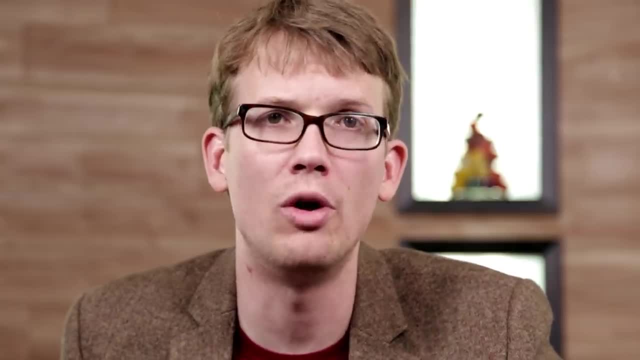 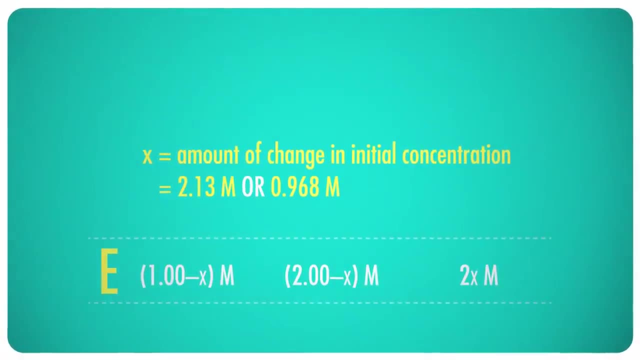 Well, neither the H2 nor the F2 could possibly lose 2.13 moles per liter when they both started with less than that already, So clearly the correct answer has to be 0.968 molar. Using that, then, we can calculate the actual equilibrium amounts for each substance.